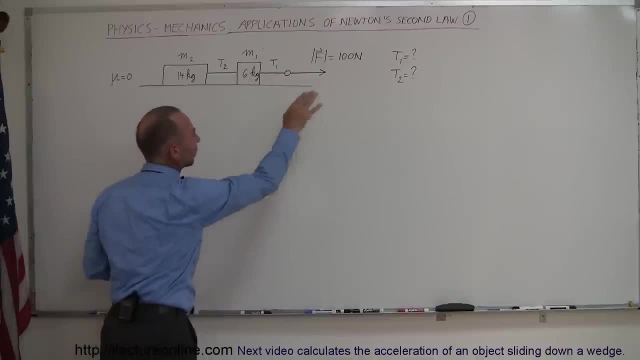 a string. The first one has a string attached with a little ring and we pull on the ring with a force of 100 newtons. This one is 14 kilograms, This one is 6 kilograms. The question is: what is the tension on these strings? Now, in order to find the tension on the strings we probably want, 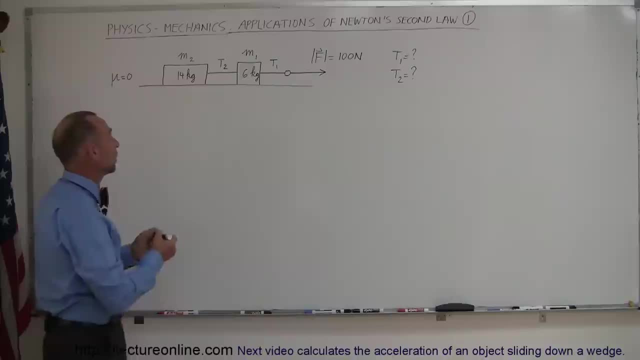 to find the acceleration of this system first, And what we could do is we could think of this as one system right here, like so, and we're applying a force of 100 newtons to the right, So let's explore also all the other forces that are acting on this system right here. 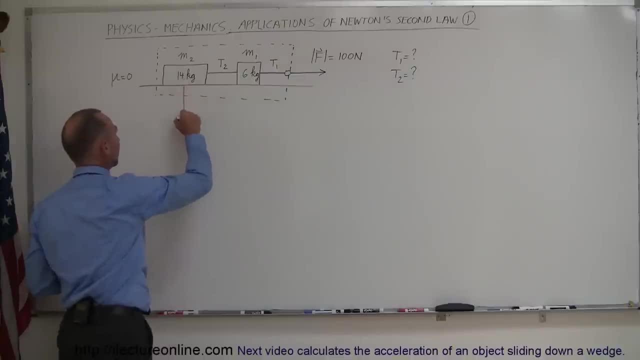 So first of all we have gravity pulling down this mass, So this would be m2g, which is the weight of the 14 kilogram mass- And then we have a force coming down this way, also due to gravity. 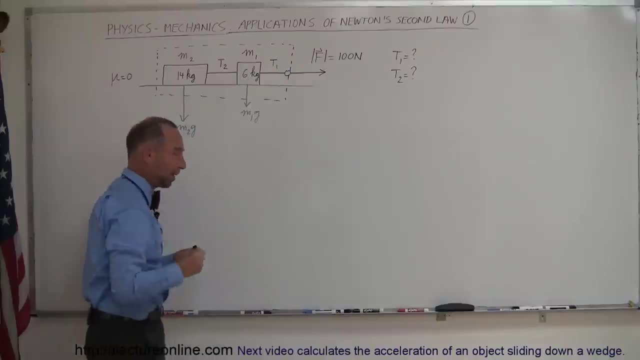 which is m1g, which is the weight of this first mass. right here, And of course, knowing Newton's third law, we can see then that there's going to be a reactionary force, a normal force, which is going to be equal in magnitude to m2g, And here we're going to have, let's call it, m2.. And 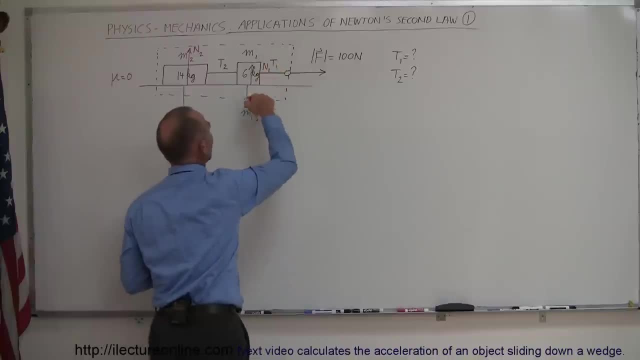 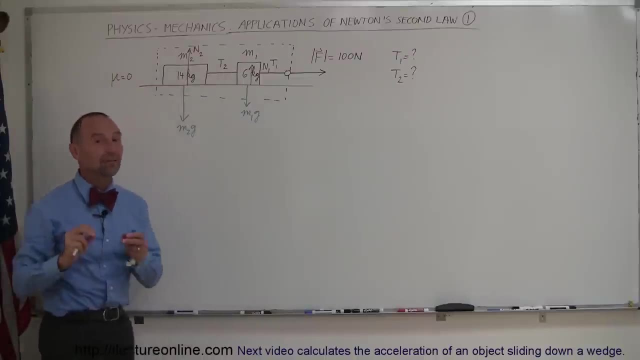 here we're going to have a normal force- let's call it n1, which is going to be equal in magnitude to m1g and, of course, in opposite direction, so that these forces cancel each other out, so that there is no net force in the vertical direction. So there's only one force left. 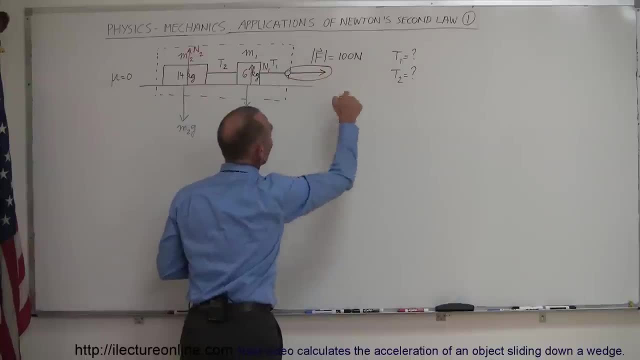 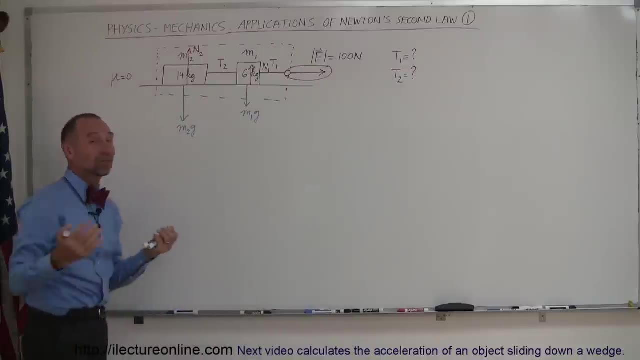 which is this 100 newton force here pulling to the right. That's the only net force on the system. Therefore the whole system will accelerate to the right At some, acceleration determined by Newton's second law. So we can start out by saying that. 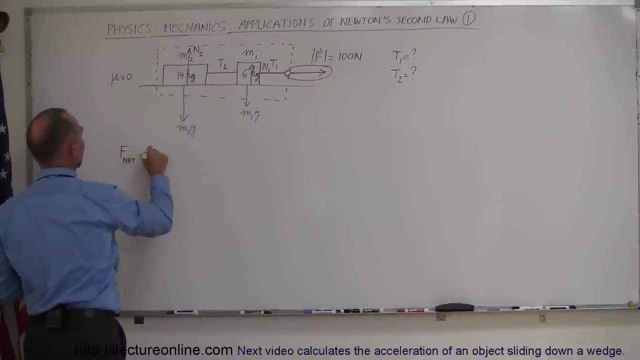 f net in the x direction is equal to mass total times acceleration. This sub t here simply means the total mass of the whole system. So therefore the acceleration is equal to the f net divided by the mass total, which is equal to 100 newtons divided by the sum of the two. 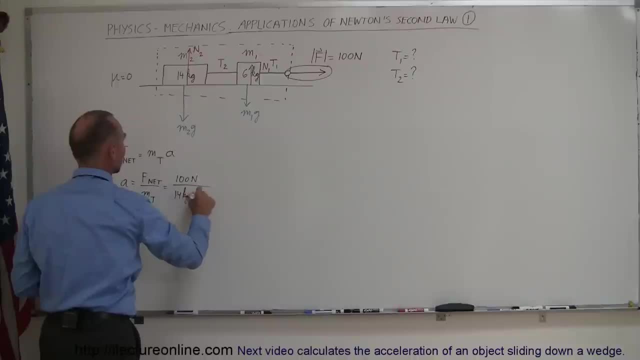 masses, which would be 14 kilograms plus 6 kilograms, And so that's 100 divided by about 20, or 5 meters per second square. So now we know the acceleration of this system, which of course also is the acceleration of the individual masses. All right, now the next thing. 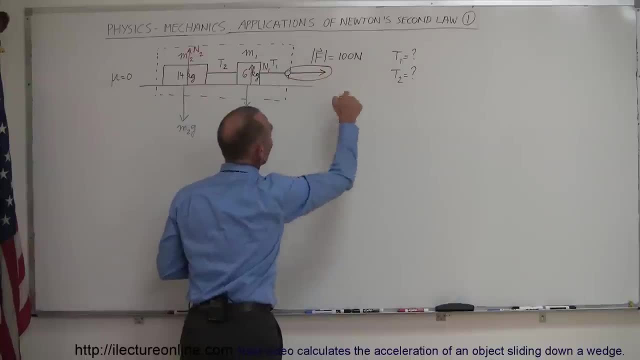 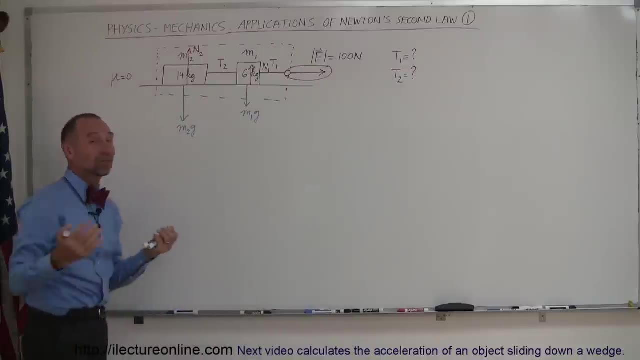 which is this 100 newton force here pulling to the right. That's the only net force on the system. Therefore the whole system will accelerate to the right At some, acceleration determined by Newton's second law. So we can start out by saying that. 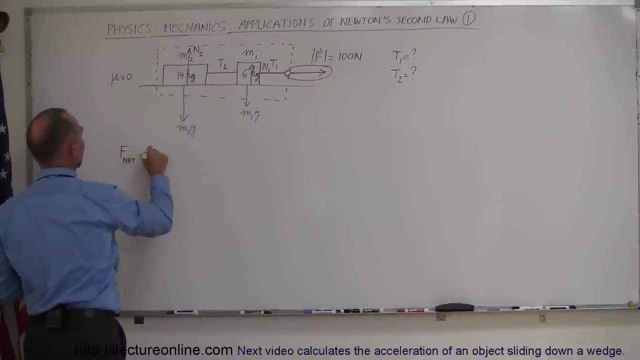 f net in the x direction is equal to mass total times acceleration. This sub t here simply means the total mass of the whole system. So therefore the acceleration is equal to the f net divided by the mass total, which is equal to 100 newtons divided by the sum of the two. 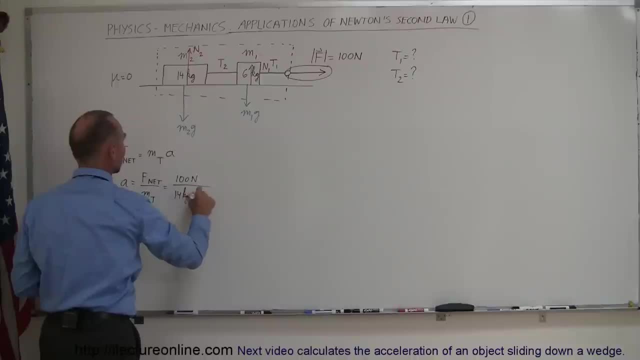 masses, which would be 14 kilograms plus 6 kilograms, And so that's 100 divided by about 20, or 5 meters per second square. So now we know the acceleration of this system, which of course also is the acceleration of the individual masses. All right, now the next thing. 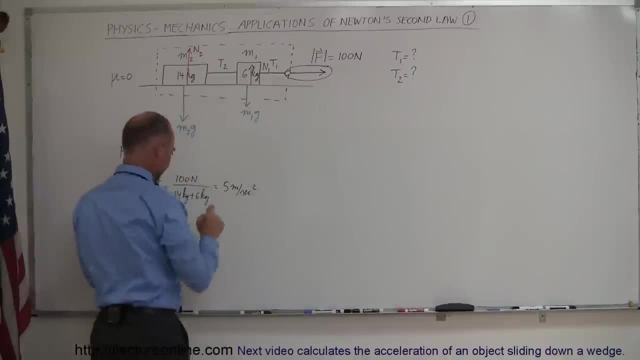 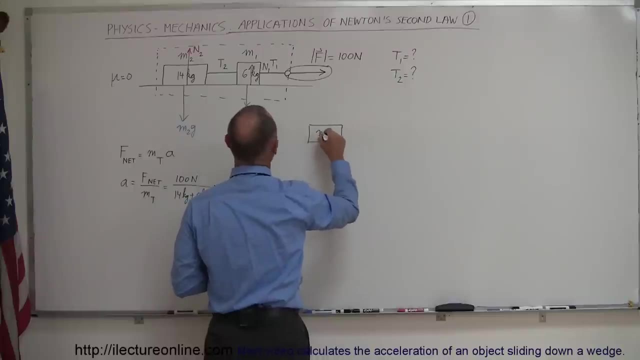 we'll want to do is find the tension here, tension 1.. And if we draw a free body diagram of the situation, we have these two masses right here, We have m2 connected with a string to m1, and then that's connected to a string. right here We're trying to find the tension over. 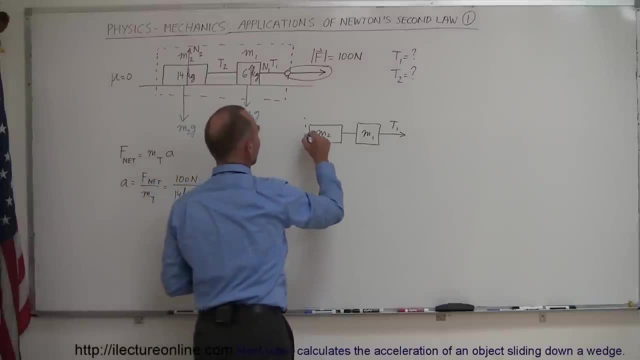 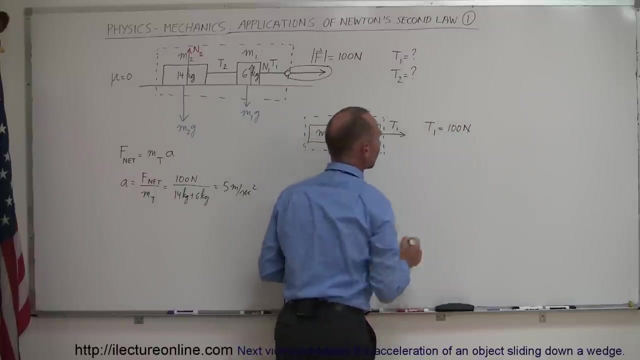 here. And of course we have a similar situation that if we consider this whole system we can see that the tension in one is accelerating the whole system. So therefore the tension one has to equal the 100 newton force right here. So we can say that tension 1 equals 100 newton. Now what would 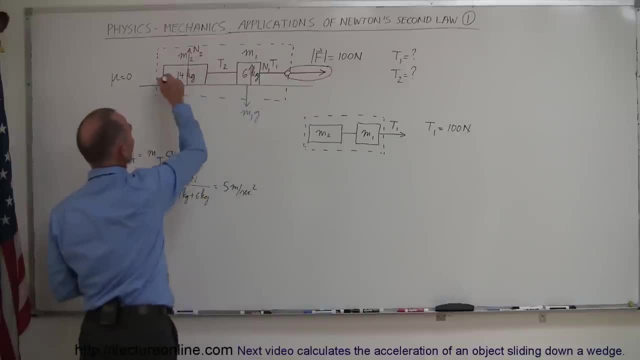 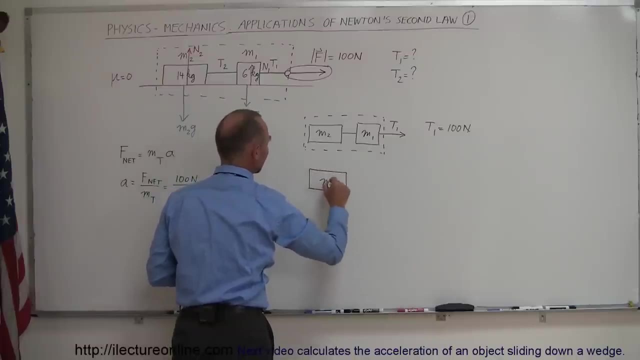 be the tension in the second string. Well, for that we're going to just simply draw a free body diagram of the second mass. So in this case we simply have the second mass right here, m2, with a string attached to it, And therefore we realize we're going to have a tension to the right. 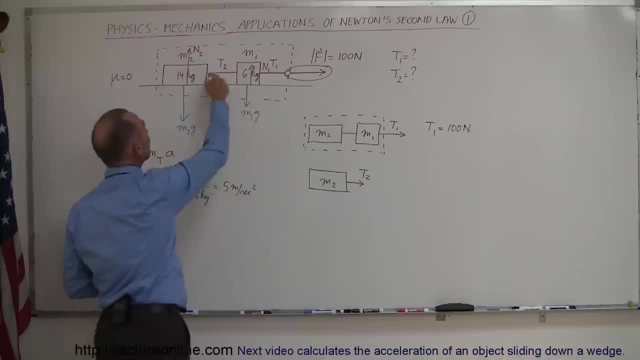 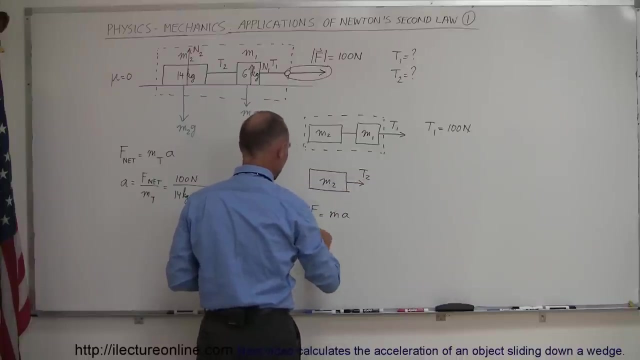 accelerating m2 to the right. So the tension in 2 only accelerates the 14 kilogram mass. It does nothing to accelerate the 6 kilogram mass. So from Newton's second law we can say that f is equal to ma. In this case of course we have the tension. Tension 2 is equal to the mass. 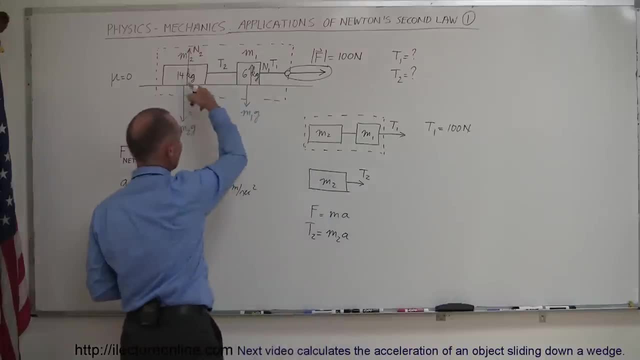 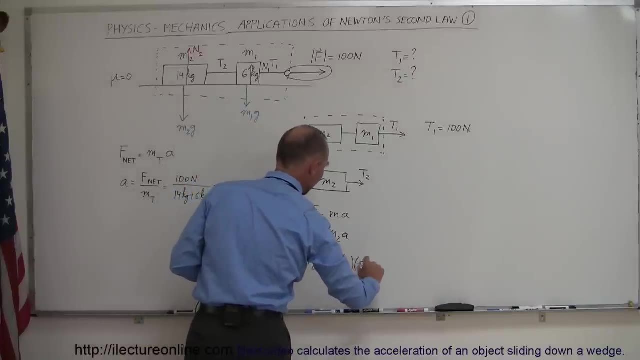 mass 2 times acceleration, which is the same as the acceleration of the whole system. So we can say that T2 is equal to 14 kilograms times 5 meters per second squared, And so the tension in the second string is 70 newtons. So we have the tension in the first string.